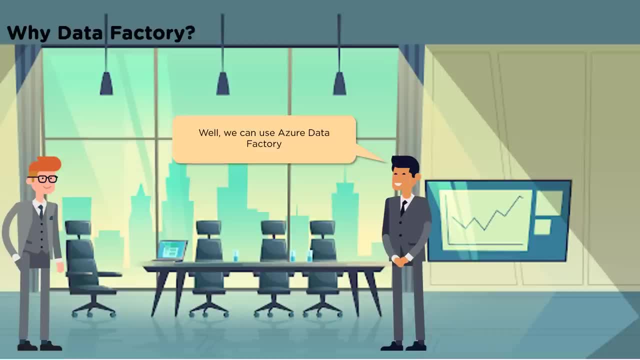 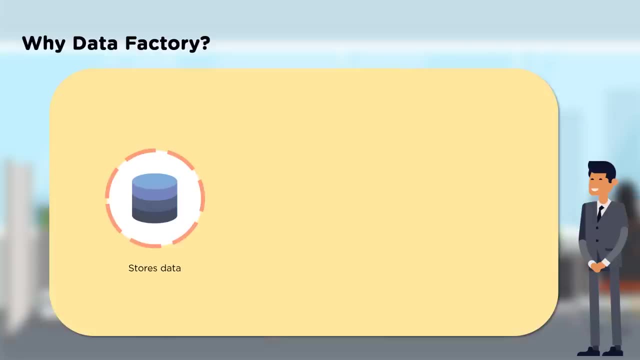 this data. So he wonders how they're going to manage that. His friend suggests that they use Azure's Data Factory. Now, what does Azure's Data Factory actually do? First, it stores data with the help of the data lake storage. Now any kind of data can be stored in the. 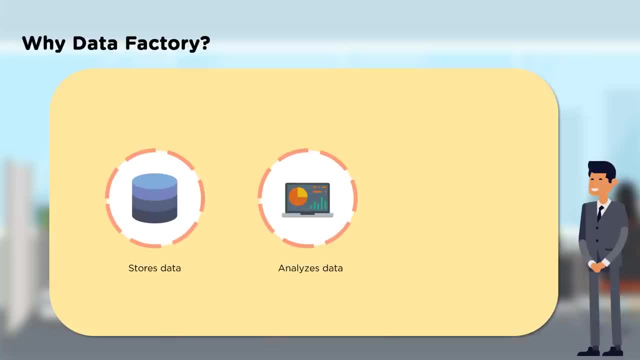 data lake storage. Then you can analyze the data, you can transform the data with the help of pipelines and you can publish the organized data. You can visualize the data with third party applications like Apache, Spark or Hadoop as well. Now, what exactly? 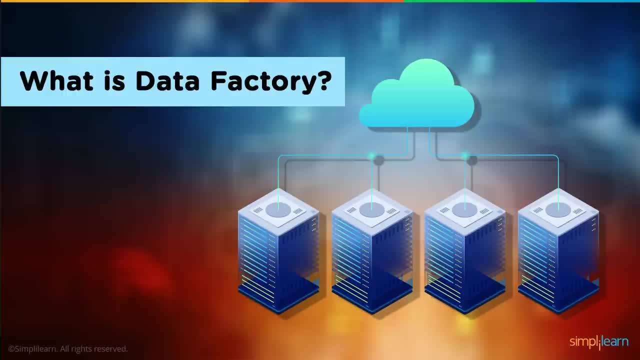 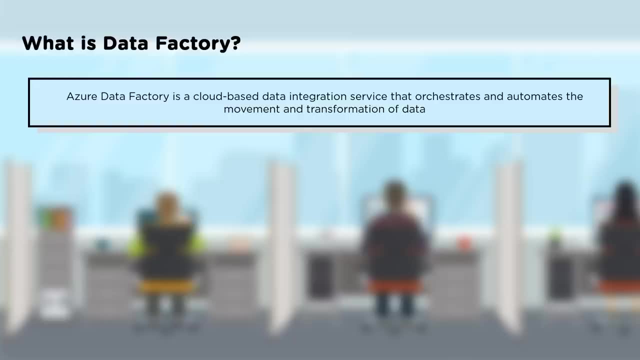 is Data Factory. So now let's have a look at what exactly is Data Factory. Now, Data Factory falls under the identity domain of services in the Azure catalog and is a cloud-based integration service. Basically, what it does is: it works on your data, it stores your data, it orchestrates. 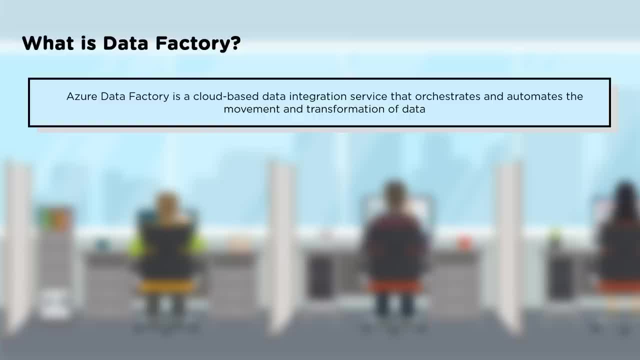 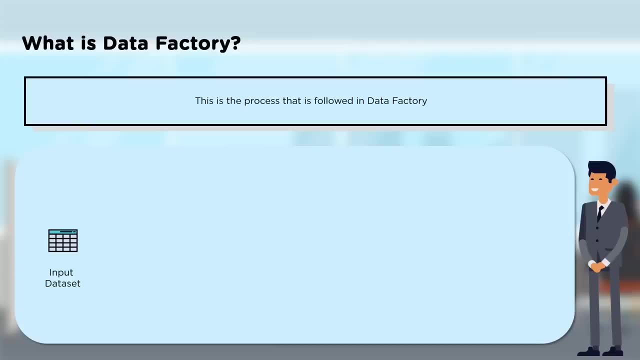 and automates the movement or transformation of data. It works heavily on the data that you store. Now let's see how it actually works, or how the flow of its processes are. Firstly, we have the input data set, which is nothing but the data that you have in the 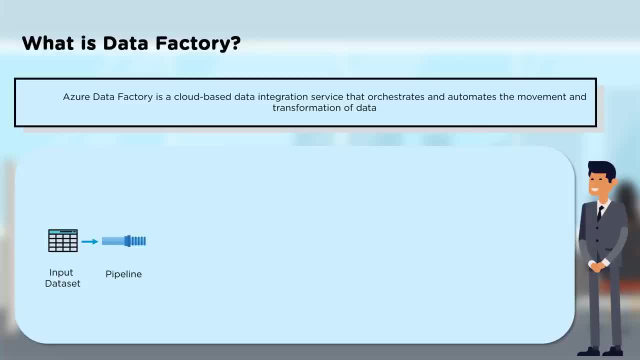 database within your data store, the one that you need processed. Then you pass this data through a pipeline. Now, what does a pipeline do? A pipeline basically performs an operation on the data that transforms it, which could be anything from just data movement or some. 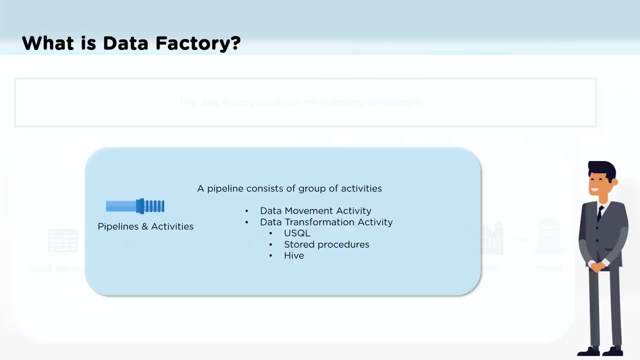 data transformation. Now, data transformation is possible with the help of USQL, some stored procedures or Hive Now. after this is done, you get an output data set. Now, this output data set will contain data that is in a structured form, because it's already been transformed. 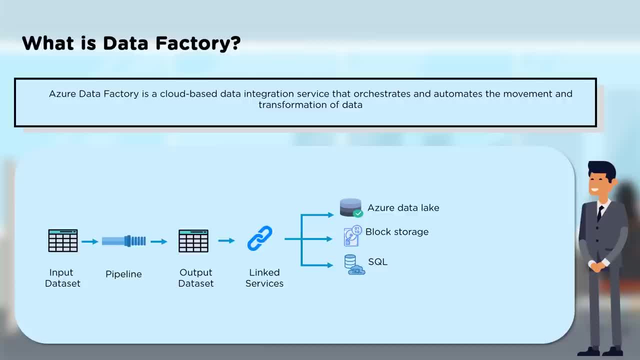 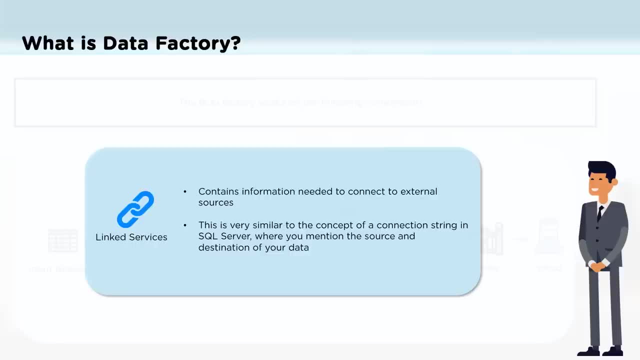 And made structured in the pipeline stage. Then it is given into linked services like Azure, Data Lake, Block Storage or SQL. Now what it does is these store information that is very important when it comes to connecting to an external source. Now, this is you know. 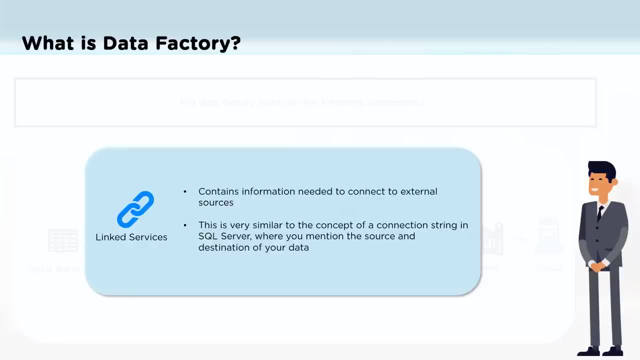 if you wanted an example. you know how. in an SQL server, you need to mention the source and destination of your data. Now, for example, consider an SQL server. So you need a connection string so that you can connect to an external device. You need to mention the stores and. 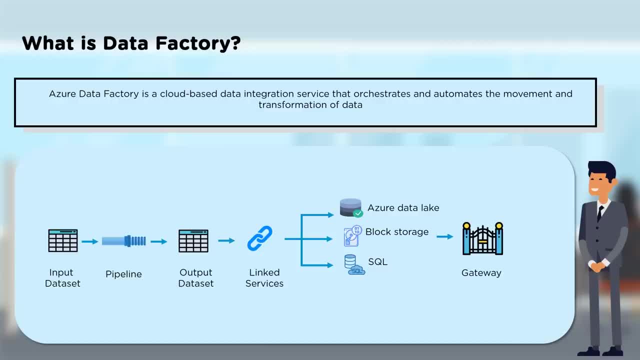 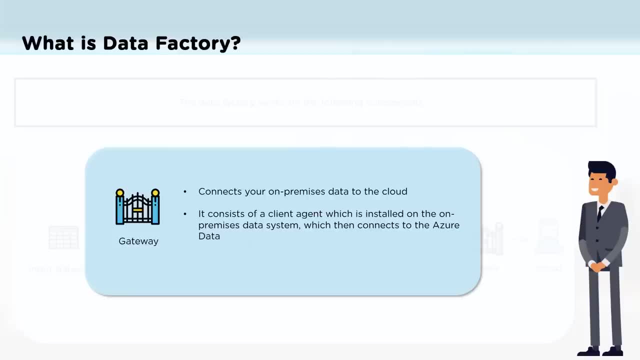 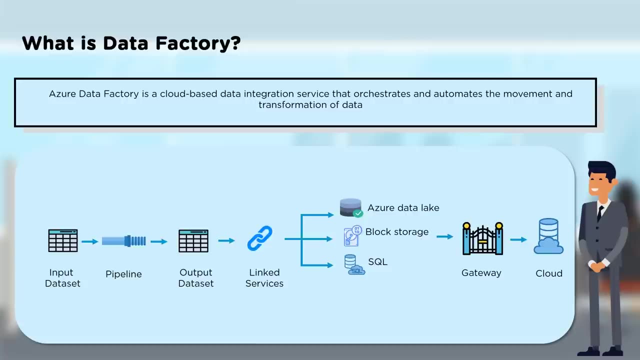 the destination of your data. This is how the linked services work. And finally, you need a gateway. Now, a gateway basically connects your on-premises data to the cloud. So you do need a client installed on your on-premises system so that you can connect to the Azure cloud. And finally, you 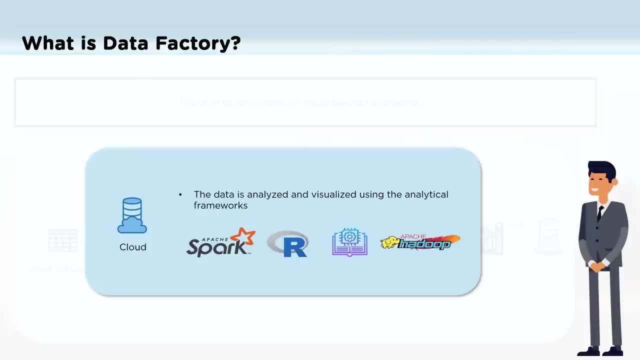 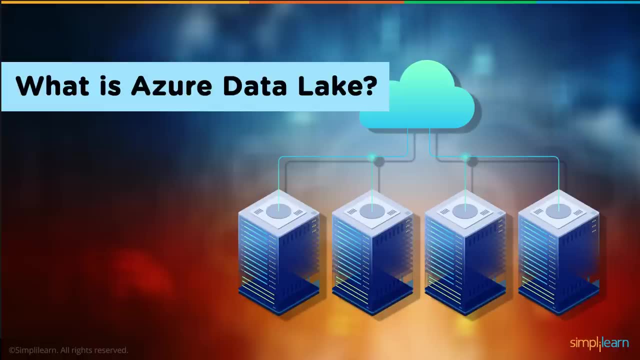 have the cloud Here. what happens is your data can be analyzed or visualized with a number of different analytical softwares like Apache, Spark R, Hadoop and so on. So all this time I've been mentioning that data lake is a very important part of your data, And 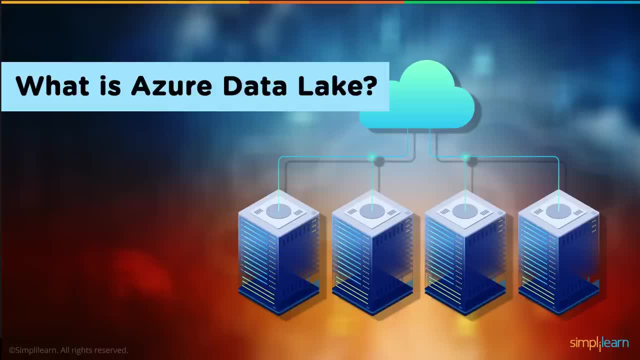 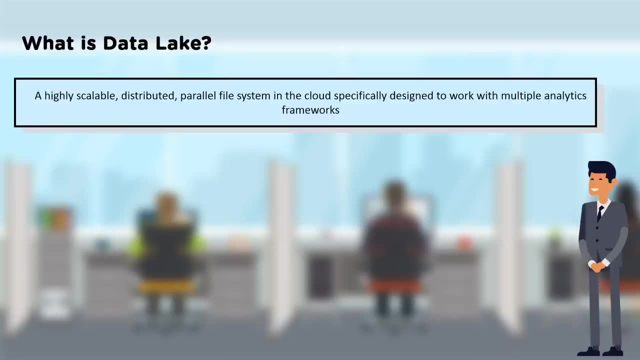 it's a very important part when it comes to Azure Data Factory's proper functioning. So now let's talk about what exactly is data lake? Now, data lake is a data storage or a file system which is highly scalable and distributed. It is located in the cloud and 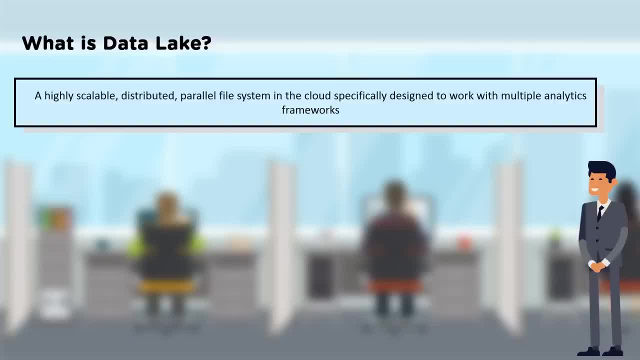 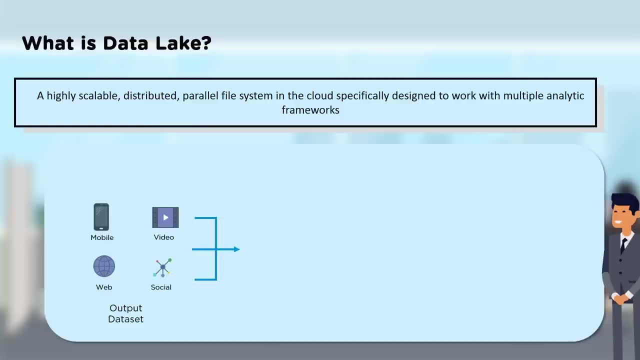 works with multiple analytics frameworks, which is, external frameworks like Hadoop, Apache and so on. So now let's have a look at it. So first you have your output data set, which is data from the mobile video, web, social media. so much more. 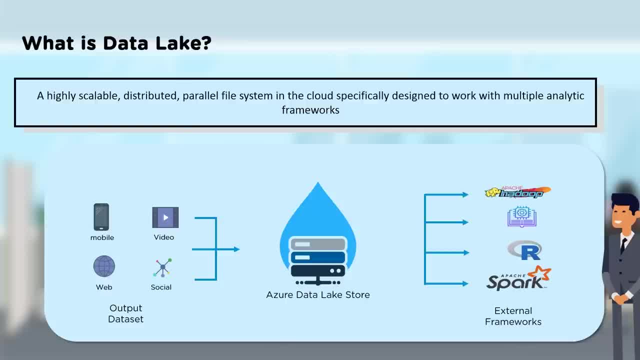 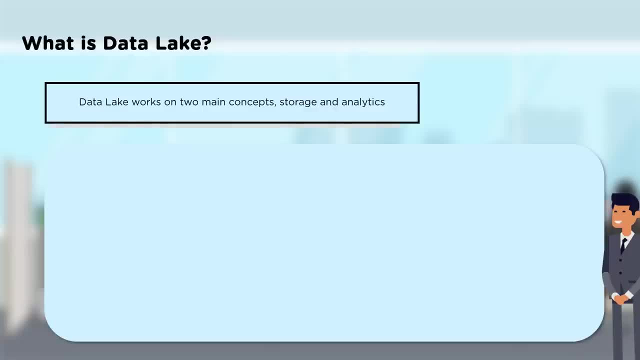 It is sent into the Azure data lake store and then it is provided to external frameworks like R, Apache and Spark so that they can be worked on. Now there are two main concepts when it comes to data lake storage, So one of them is storage and the other one is analytics. 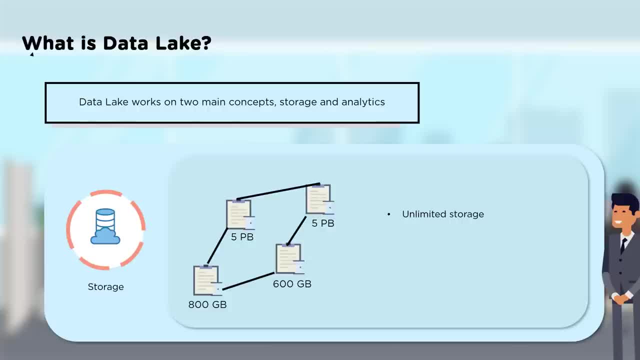 Now, storage is of unlimited size. It can be petabytes, terabytes, gigabytes and so much more. It shows a wide variety of data. It could be unstructured or structured data, and it can store really large files. And another concept when it comes to data lake is analytics. Now how it works Now. 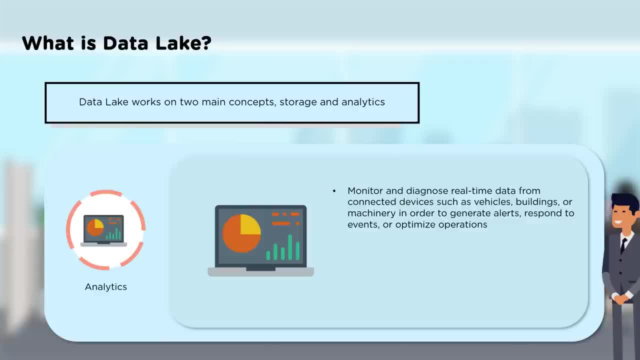 here are two examples of how analytics works when it comes to data lake. Now, when it comes to analytics, you can monitor and diagnose real time data, For example, data that you're getting from vehicles or buildings. These can be used to optimize how they work. respond. 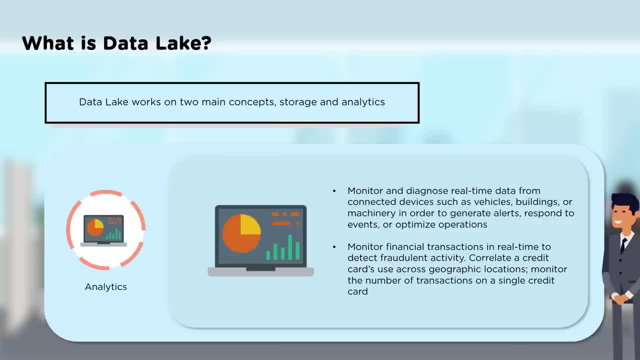 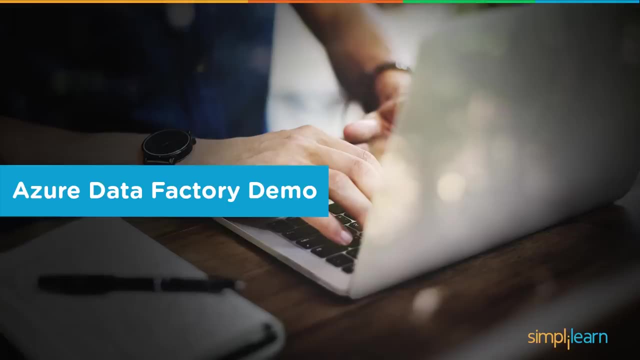 to certain events or generate alerts in case something goes wrong. Then you can also identify fraudulent transactions on your credit card, or you can identify the current, The geographical position of your card, perhaps monitor how many transactions have been taking place on that card, and so on. So now we're going to have a look at how we can use the. 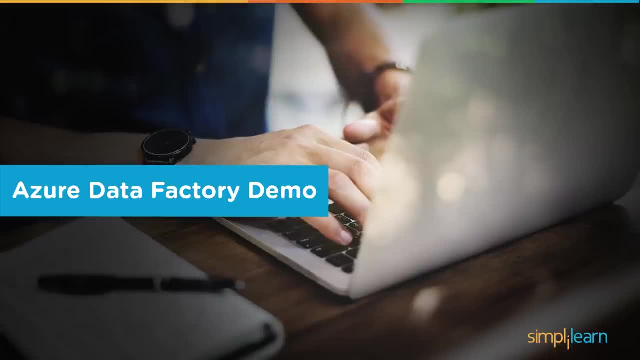 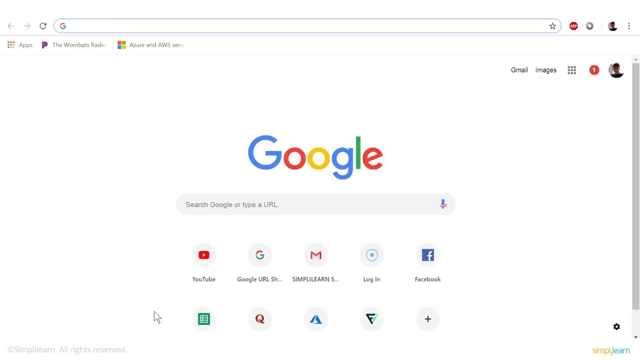 Azure Data Factory to move data from an SQL database to a blob storage on the cloud. So here's what we're going to do. So, first off, to make a database, what you're going to need is software known as SSMS, So you can find it on Google. It's called. you just need to. 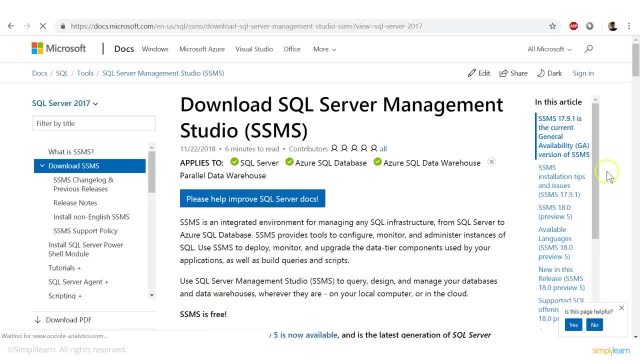 Google it, SSMS, The first thing you can take here and there you have it, So you just need to click here and download the file. I have already downloaded the file. Basically, you are going to create a database which we'll be transferring to the blob storage. 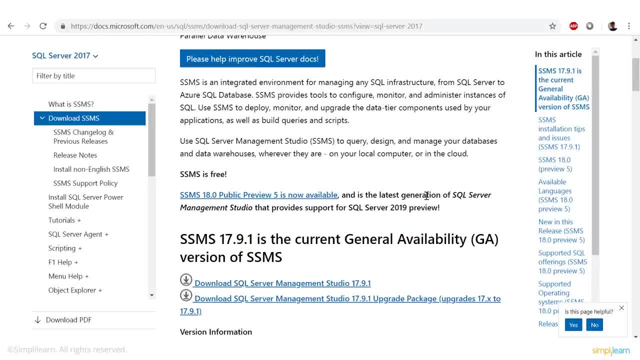 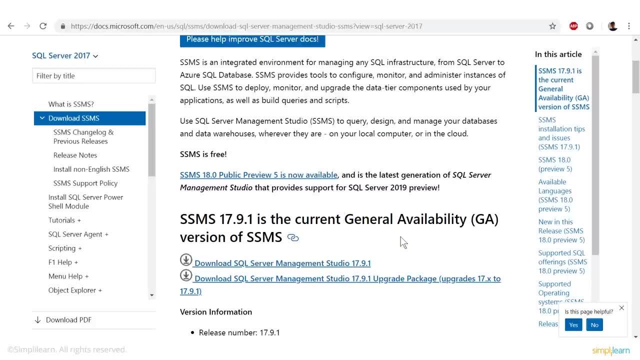 this will take about, depending on the computer speed, pretty long or little to no time. I have already downloaded the process. The process is very simple: Just directly go and say Yes, yes And finally, once installation is done here, what we are going to do is go into the. 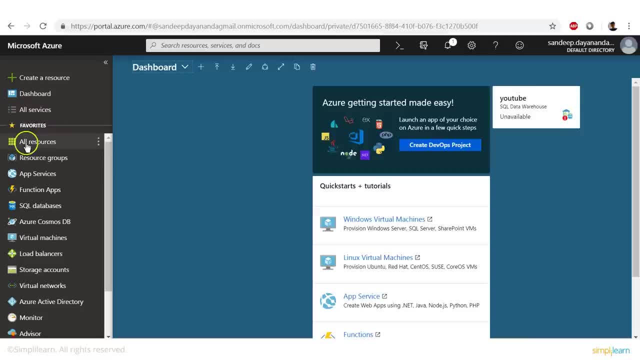 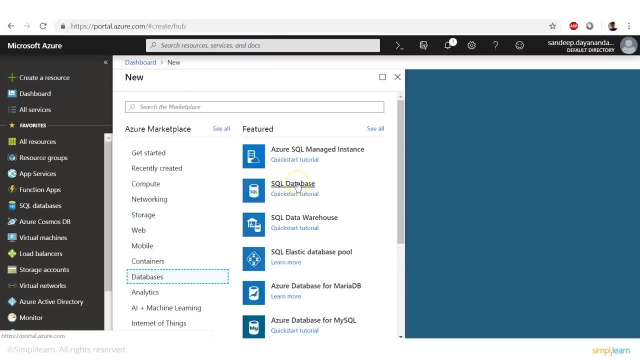 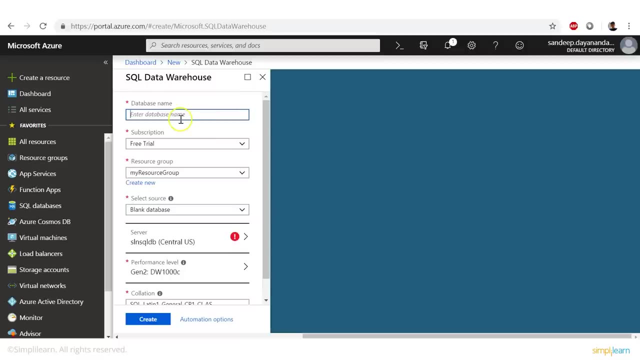 dashboard of Microsoft Azure here and we need to create a data warehouse. So you go into the sources and create a source, go to database and select SQL data warehouse. there we have it now. it's very important that you remember the names of the service, of everything that you're. 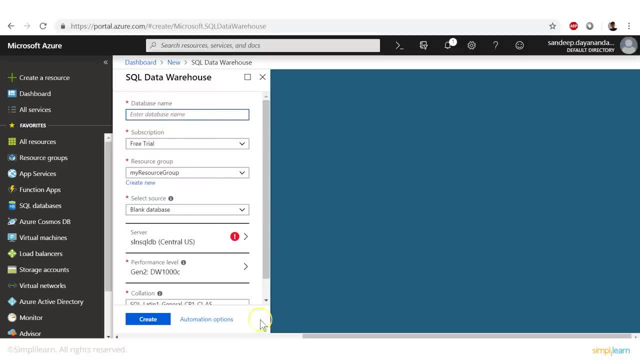 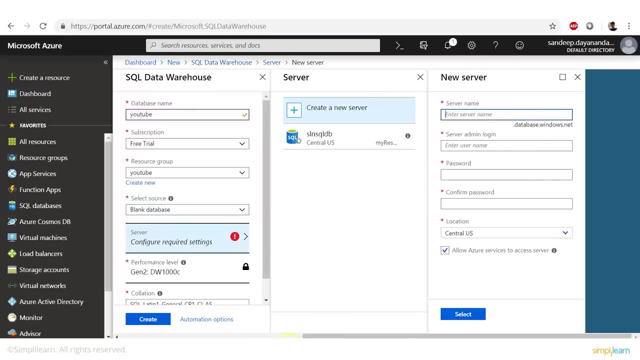 going to write here, because each of these become very important later on. so I've already set up a possible set of names: YouTube. it's free trial. the source is already created. blank database- the server. we need to create a new one, so we'll name it as YouTube server. 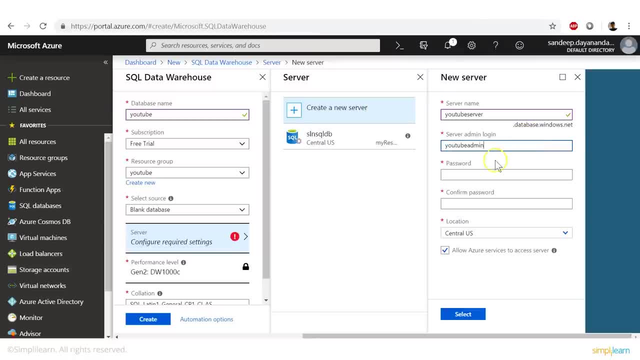 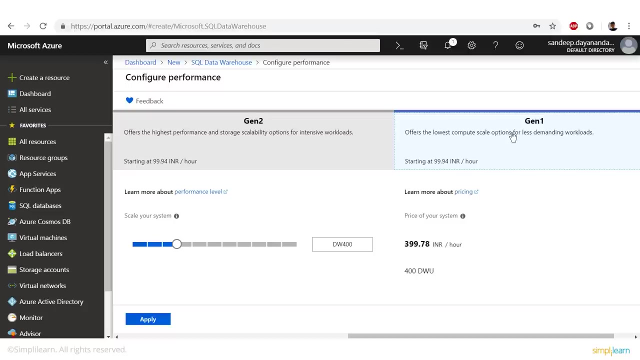 YouTube admin as the server admin, login the password as right. the location does not matter. okay, that's done. now, here the server is done and here we need to change how much you want, the lowest, I mean how much computation you want, how much did workload, how important your workload is. so we'll put it at the lowest, since you don't require. 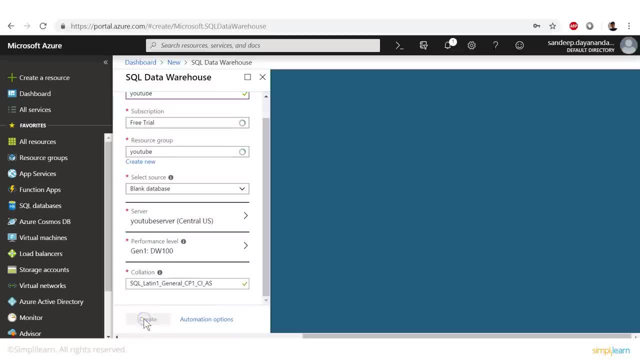 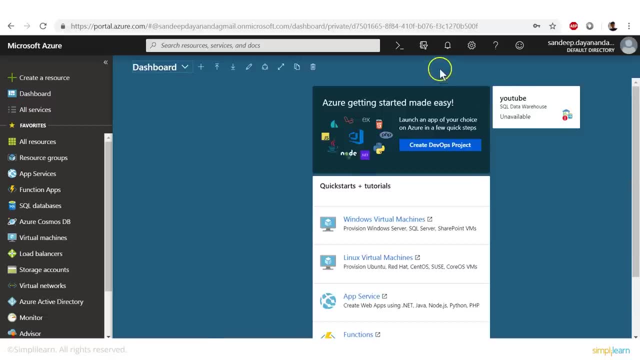 much. we'll apply- the rest is normal- and create. so now we're creating an SQL data warehouse, so we'll wait. so now the deployment is done, so we'll go to the notification and and go to the resource here. now this is done, so we'll go to the. 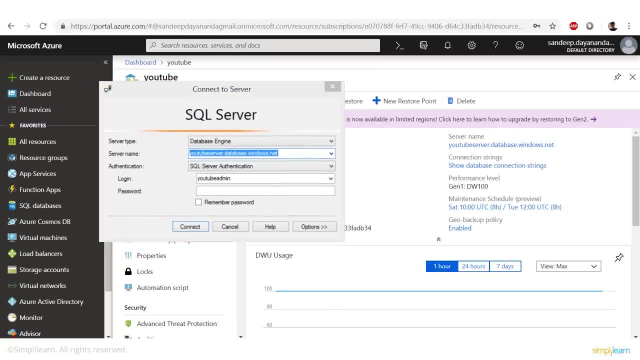 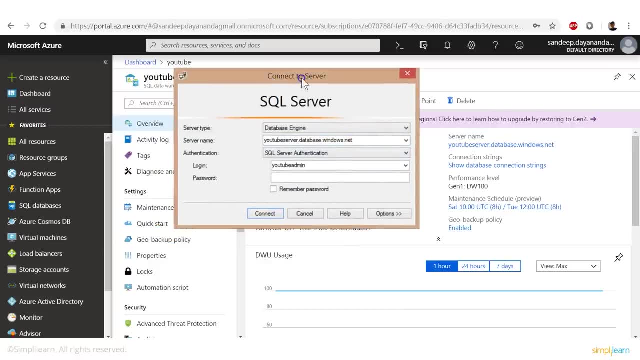 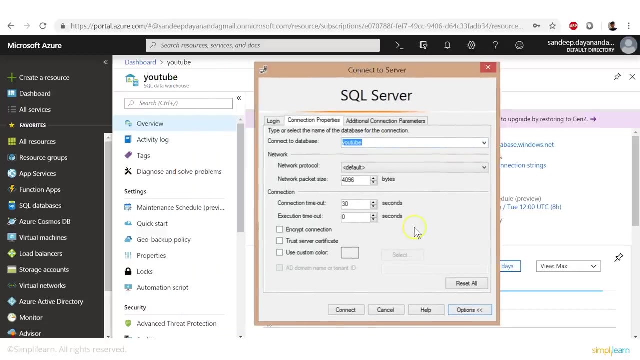 SSMS, which I've already opened here, and then go here and copy this, paste it here as your authentication login, which details we have already stored here, which is admin, YouTube admin, and the password which is also given there. right, good options. you go to the database name, which is YouTube. everything else is. 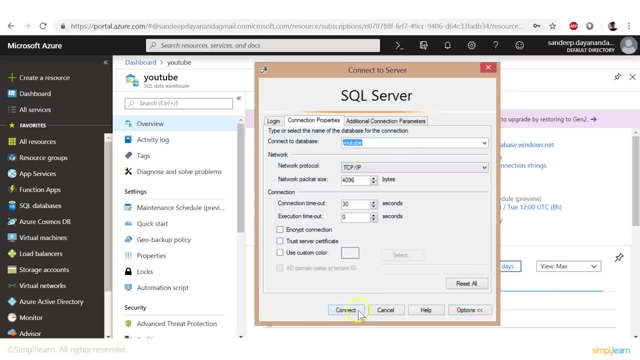 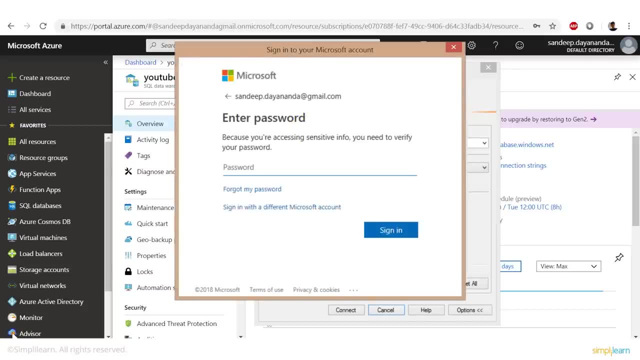 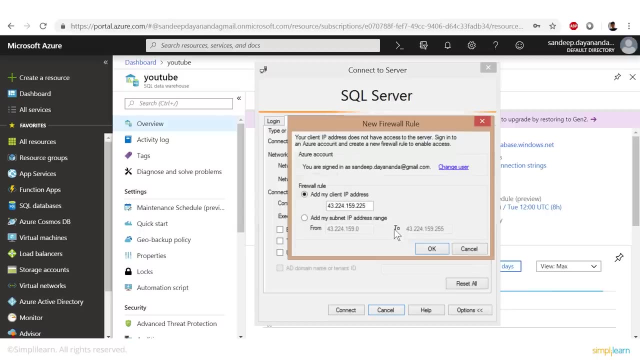 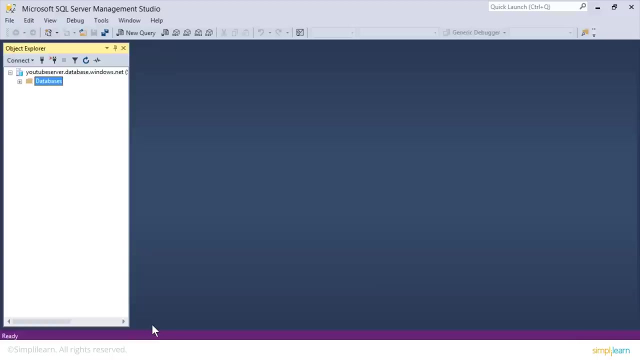 there. you need to change it to TCP IP and connect. we sign in. we'll add the password you can. we're going to sign in now, right? so now that that's completed, you can see that this is what will pop up. so this is the name of the server we've given, as you saw earlier. we're going to databases. 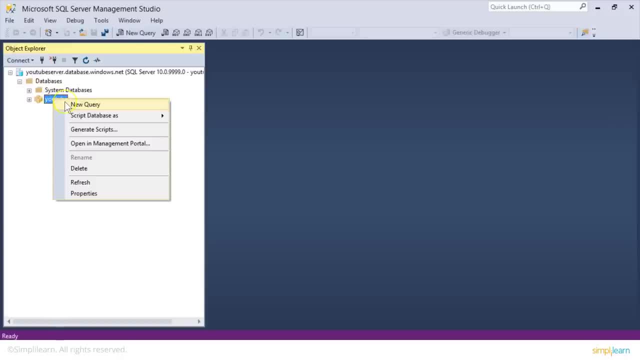 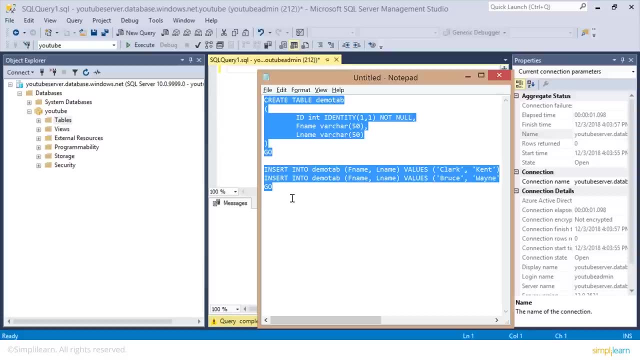 and here you have the YouTube database that we just created. right click this and add a new query. I already have a code for this program. it's a very simple program, so let's go ahead and paste this. if you need the code for this program, let us know in the comments below it's. 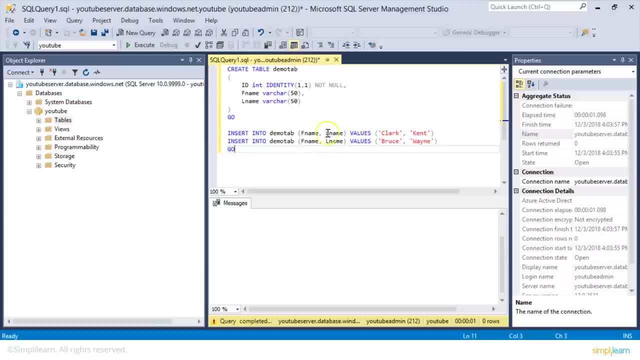 very simple. what we're doing is creating a table, called demo tab, with first name Clark Kent, last name is Bruce Wayne, and the table that's created will have these two rows. so now we're going to execute this. there you have it. two rows have been affected, so now let's have a look at our table. 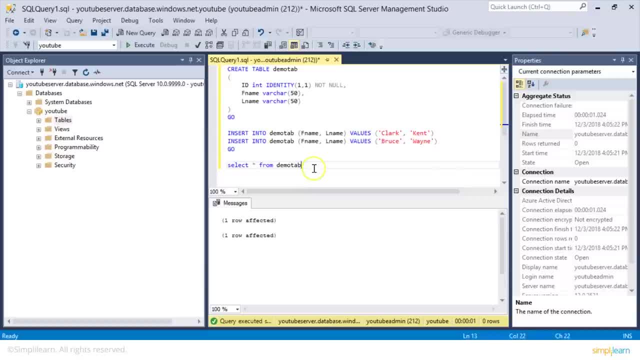 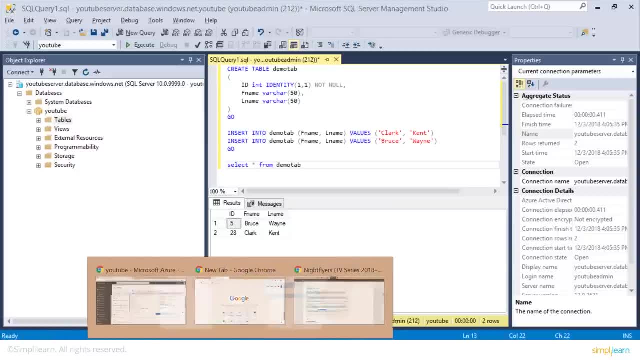 execute this line and there you go, the tables here. so now that this is done, we are going back into, as you're back, and we need to create a storage account. so that's where the storing that, the blob storage, is going to happen. so we're going. 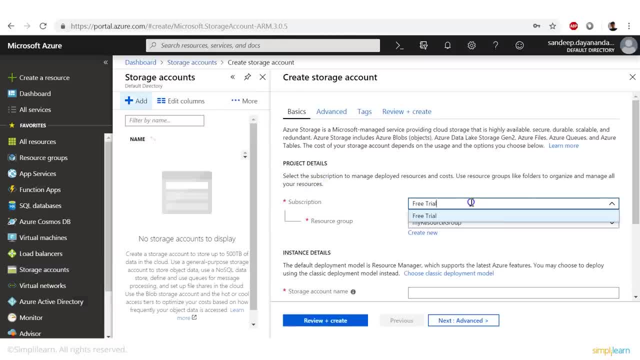 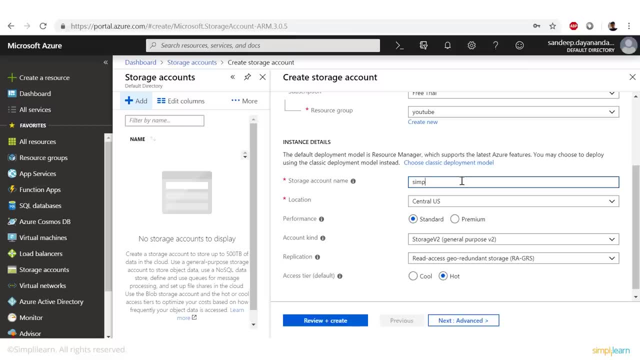 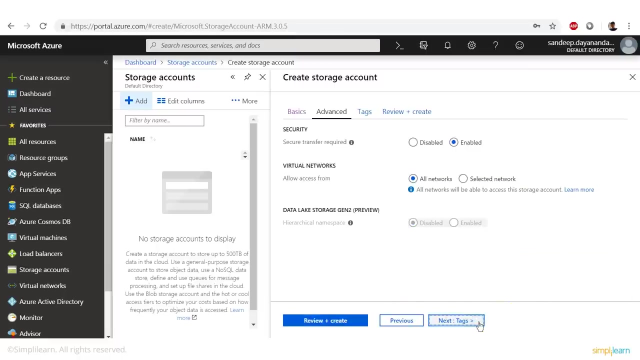 to storage accounts and click on add. so here it's a free trial resource. group is YouTube storage account. name is the store, that's okay. yes, performance is standard general purpose locally, since you don't need very reliable, at least for this one. advanced is fine view and create. that's done and 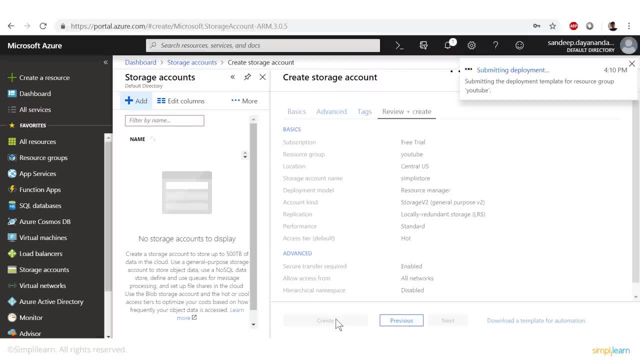 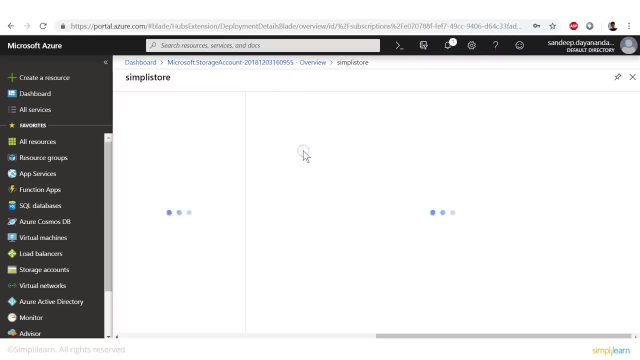 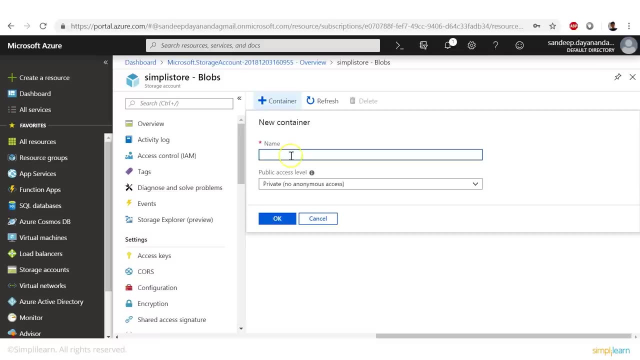 we create now, we'll wait for the deployment to finish and that's it. the deployment is done, so we'll go to the resource and go to blobs. so this is where the storage is happening. we need to create a blob, simply blob, which does not exist, and okay. 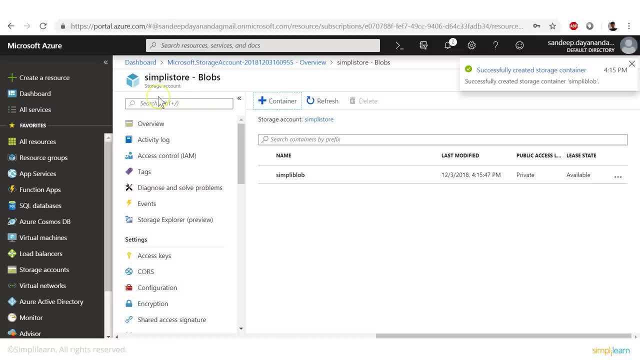 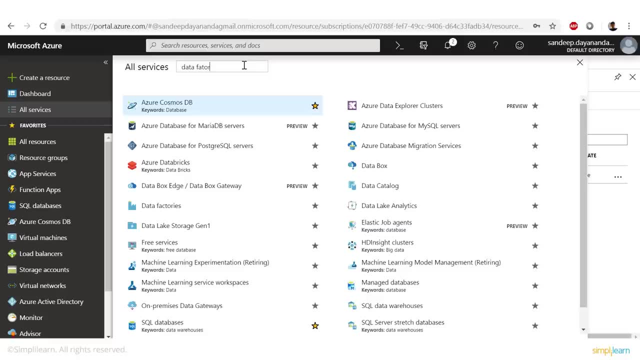 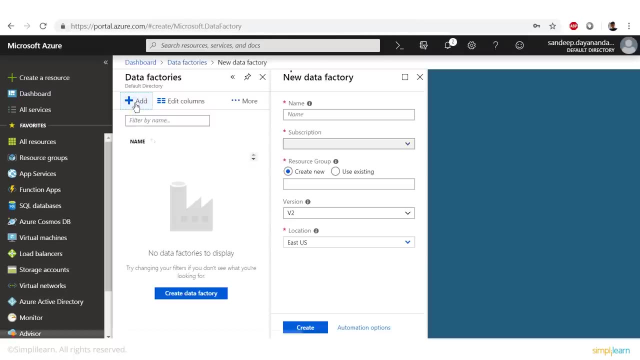 it has been created. now for the next bit. we need to create the data factory now. so we go to all services, search for data factory. you press add. so here we free trial. use existing which we have- YouTube, ECS- and create. so now we've created a new data factory. now we'll wait while it's being deployed. so now, 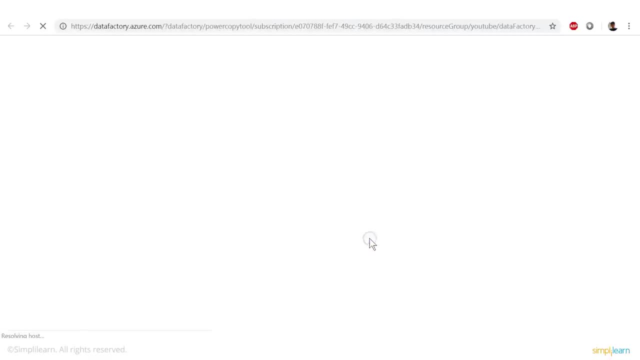 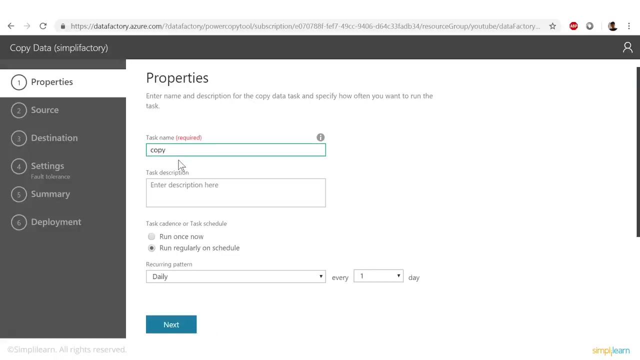 it's created. so we'll go here and here we click on copy data and this opens up: name it now, description and once now, once now, okay, alright. so we press next. so we need to connect to a data source, so so what you need to do is select a. 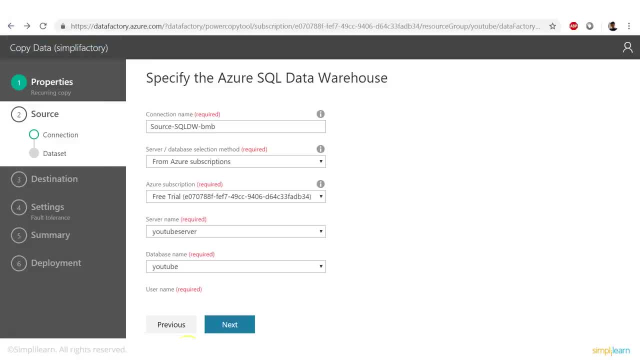 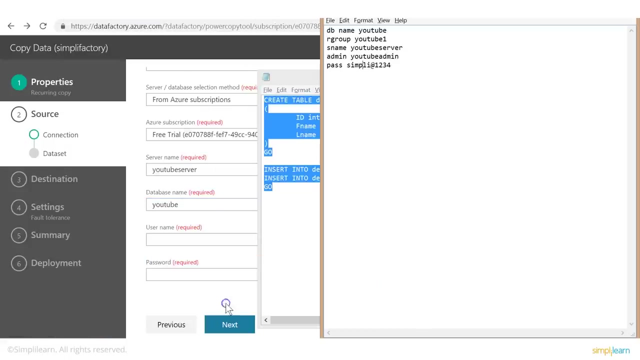 secure your SQL Data Warehouse. so once again, previous here we select games your SQL Data Warehouse. go here. search for source subscription free. try here. YouTube server and the database is YouTube. You also need to provide your username and password. I've saved it here: YouTube admin. 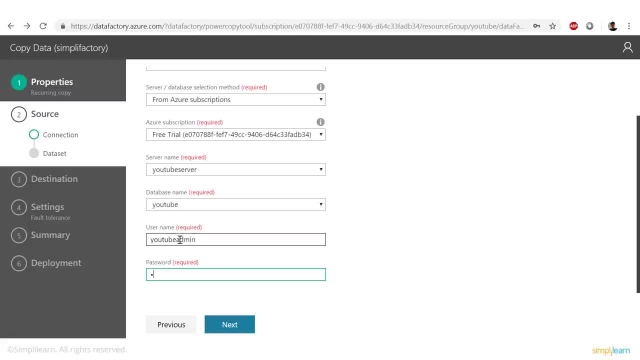 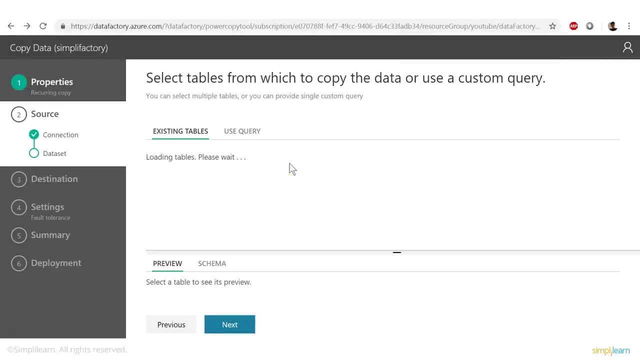 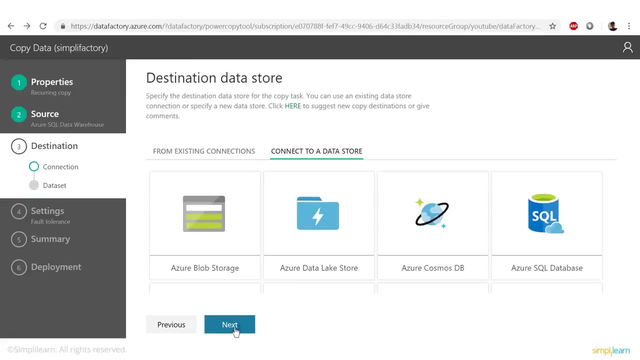 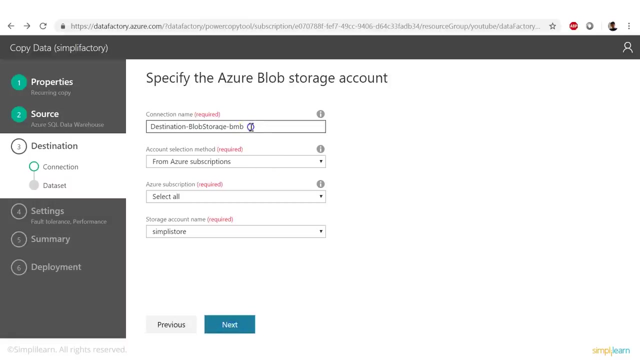 Right, Okay, now we can select the table, which is demo tab. Next, Next And now for our destination. So where are we going to connect this to? We're going to Azure blob storage. Next Destination, JavaScript solution, free trial And simply store.